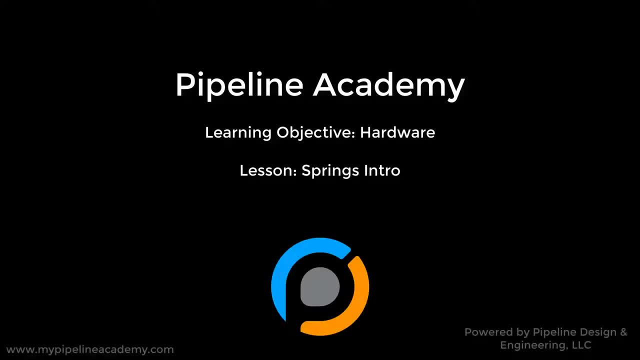 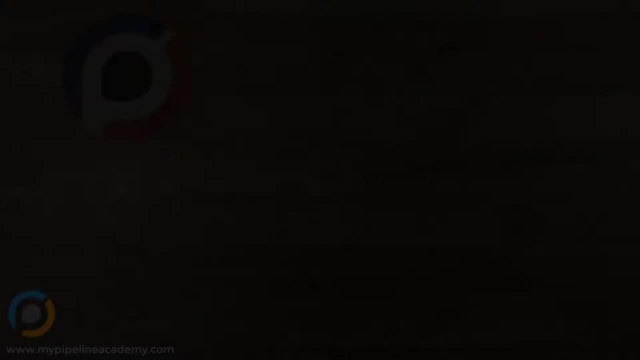 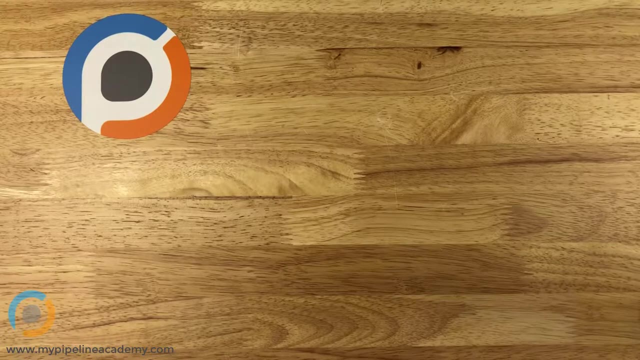 What would you do if you had an application in which you wanted to push on something or turn something a little bit and then have it move by itself, without any input from you, back to that original position? What hardware would you use for that? Well, today we're going. 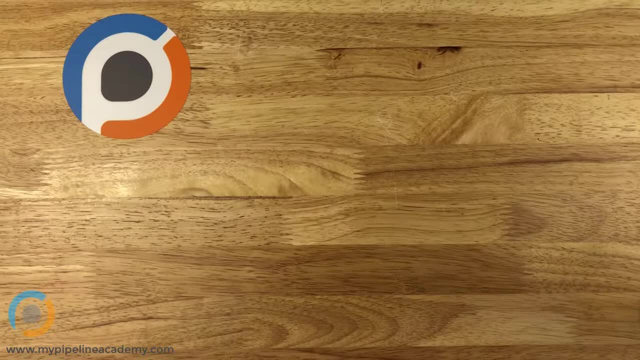 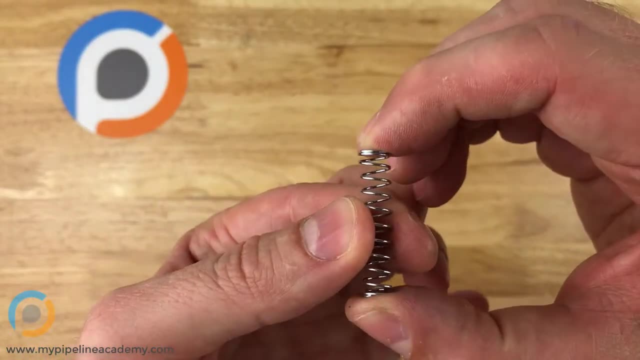 to talk about springs, and there are a few different kinds that we're going to look at. The first one is this one right here. This is called a compression spring- Compression because you you compress it in order to, to store energy in it. Springs are kind of energy. 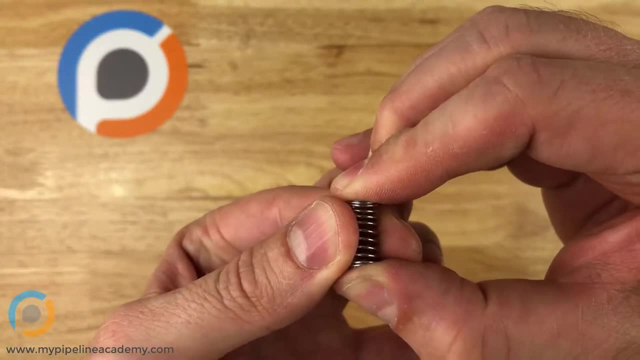 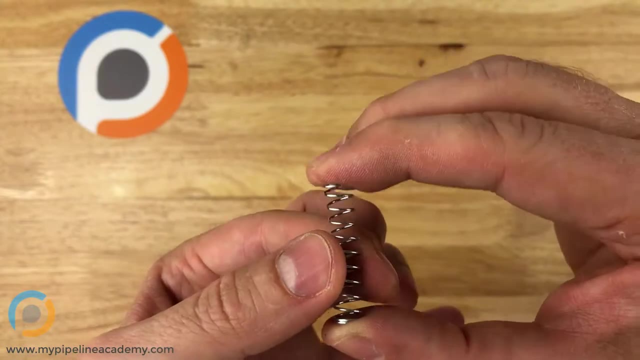 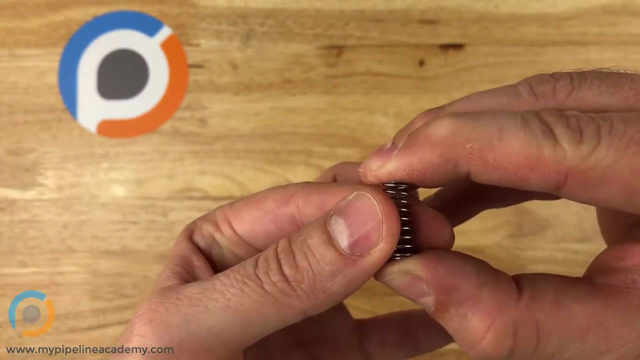 reservoirs right. You push it to put energy into it and then when you release it, that that energy is spit back out at you because it has been stored in here and you know while you're pushing on it and holding it there requires a force to hold it compressed and for some applications you might. 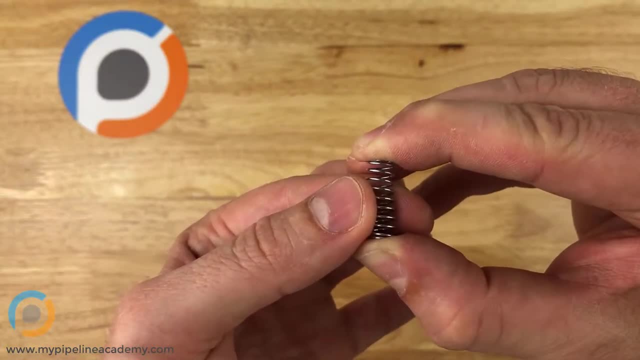 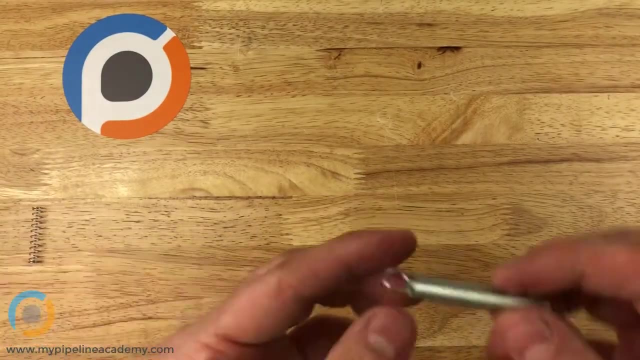 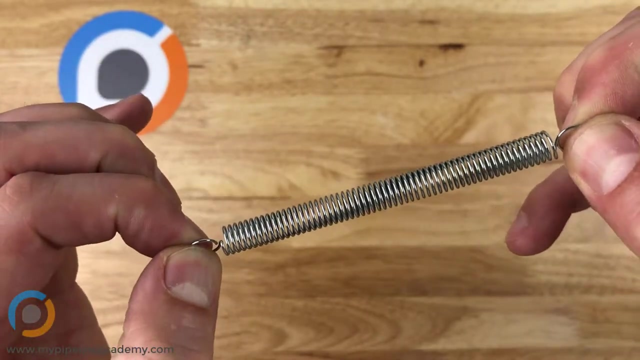 want that to be the case. You know, applying some usually small amount of force on an object can consistently or constantly, So that's a compression spring. and we have here a an extension spring, and called an extension spring because you extend it in order to put energy into. 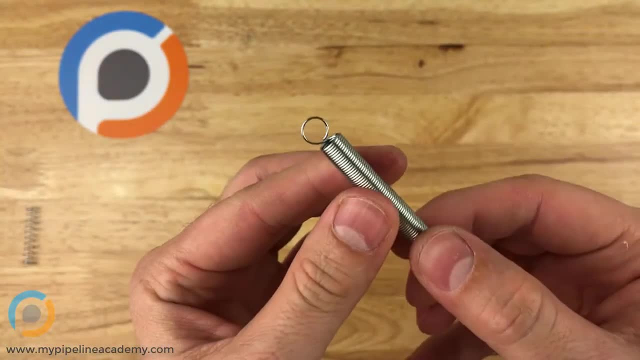 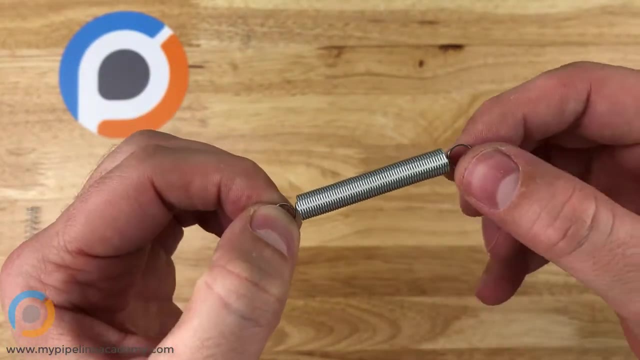 it and then it contracts. Extension springs: have these, these loops at the end so you can loop them around something. You might have a dowel pin on this end and maybe a screw goes through on this end and you can pull them apart like that. Next, we have a torsion spring. 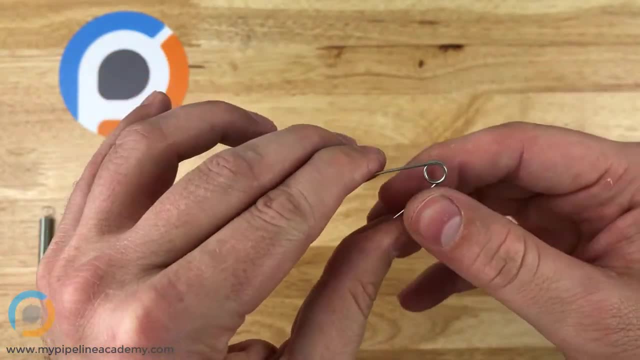 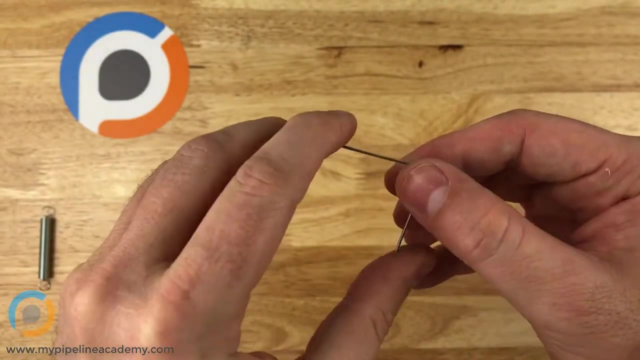 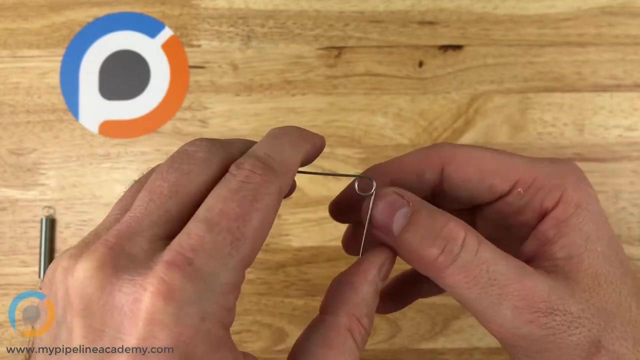 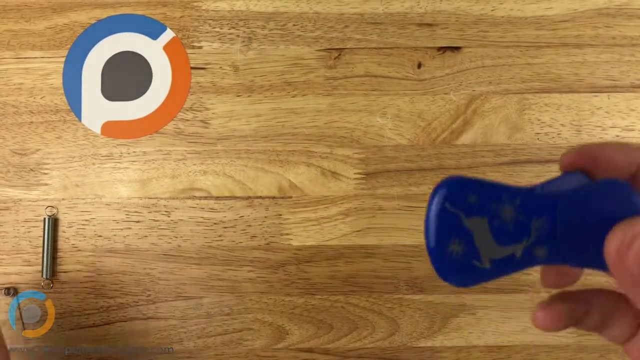 This guy here- and torsion springs. unlike the compression or extension springs, they, they, they hold rotational energy, so they produce rotational motion. you can see, you know, with my fingers right there rotating about the axis that goes through the, the center coil there. A really common example of these is these little refrigerator magnet clips. 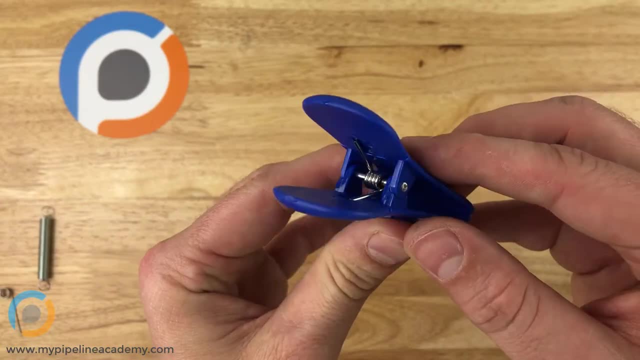 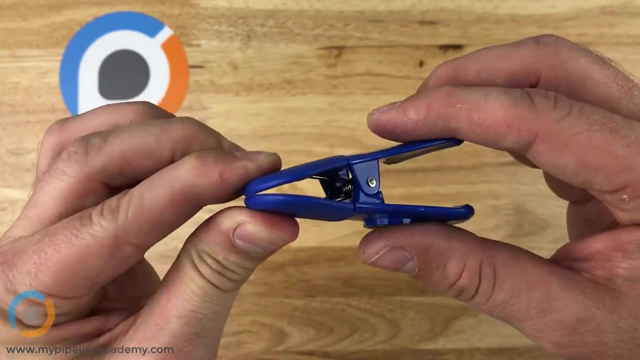 in the middle of the table. They're called torsion springs, and they're called torsion springs. You can see inside, there there's your torsion spring. Let's see here. you can see it flexing and it produces a rotational motion. Now, some of you may look at this and think that it doesn't look. 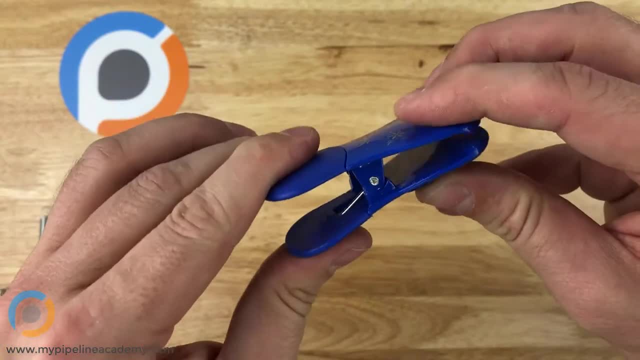 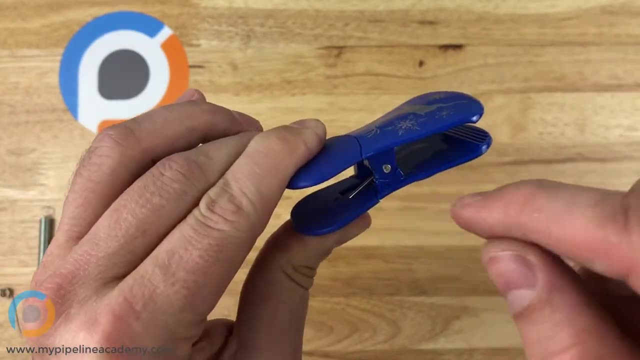 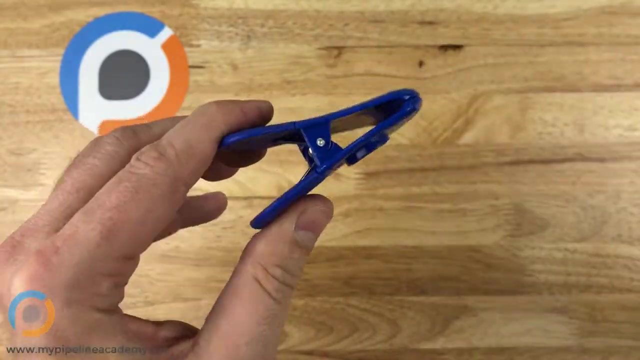 like it's rotational. but if you look at the, the rotation of these tabs there, they are rotating about an axis, The axis that you know goes through the center of that, that spring coil. So torsion springs produce rotational motion. We had an application here. here's another example of a 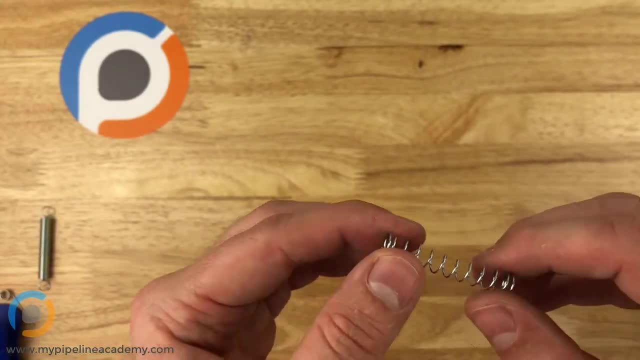 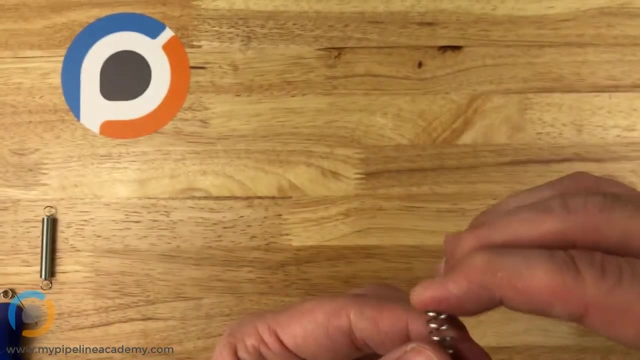 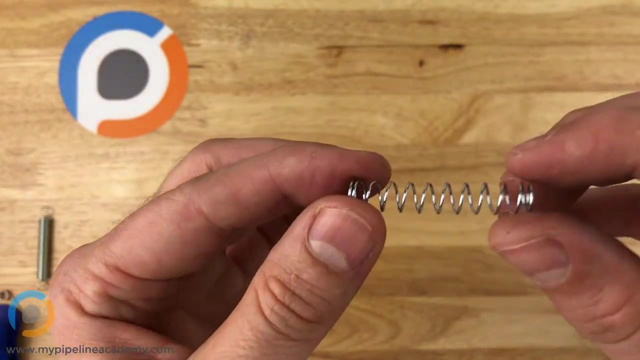 real world example of how you might use a spring. We had an application for which we we wanted to be able to push on something with up to two pounds of force and we wanted some kind of visual cue to the user that that if two pounds of force was exceeded. Now these springs, they have a what's called a. 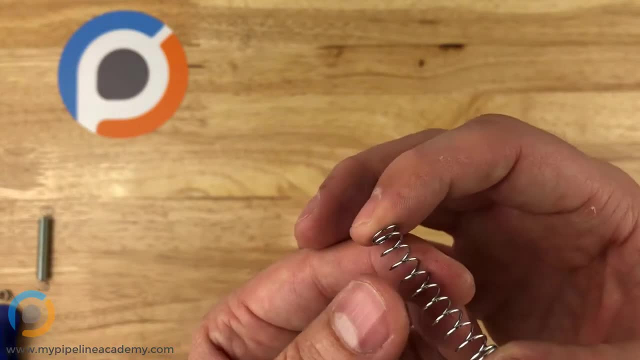 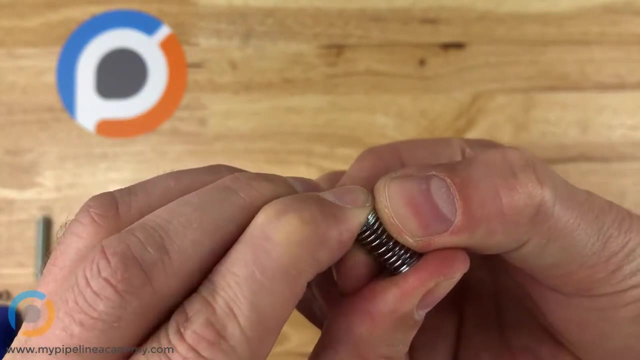 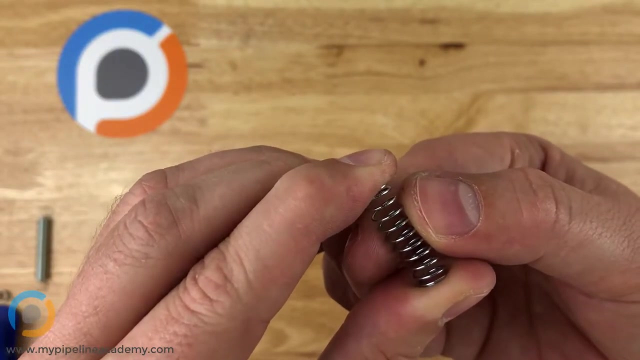 spring constant. A spring constant will allow you to very simply calculate at what amount of compression you reach a certain amount of force. So you know, if I compress this half an inch, how much force am I getting back out? How much force is the spring pushing on my fingers with? If I do, if I go a full inch now, how? 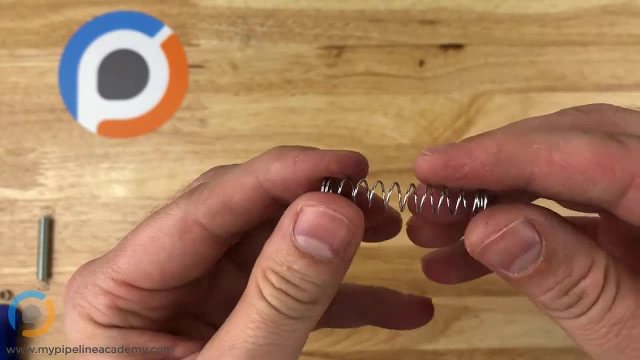 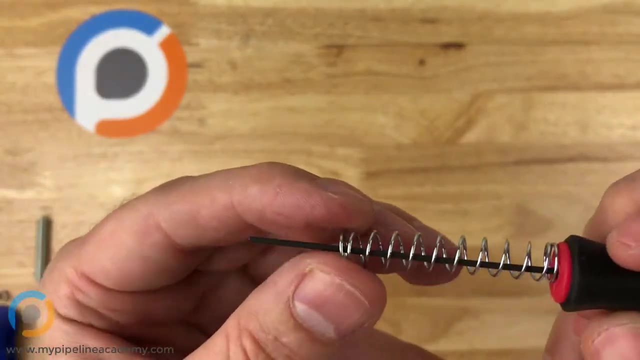 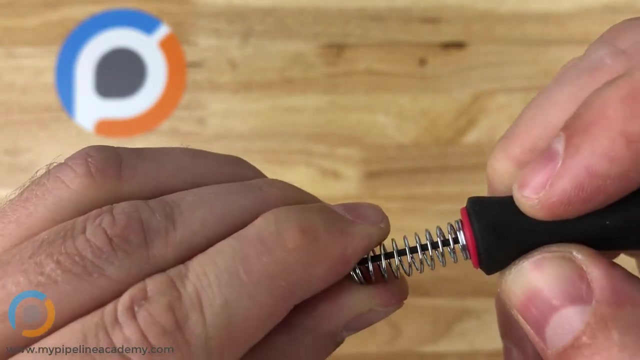 much force is the spring pushing on my fingers with? So we had this application where we we wanted to push here something like this. We wanted to to push with: uh, that's not being held that well, yeah, that's close enough- with with no more than two pounds of force, and once we reached two pounds, we wanted some kind of visual indication. 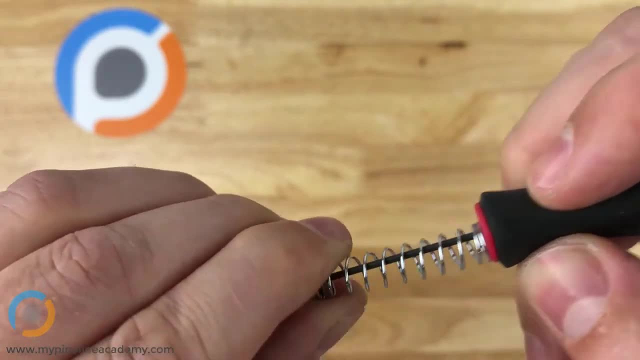 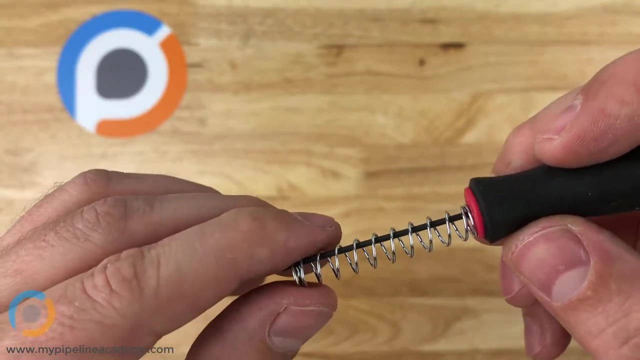 that two pounds had been reached, so that the user would not push any harder than that. Now you could implement- you know- some kind of force gauge in there, some kind of like load load button cell, but that's expensive and you know pretty high-tech solution. 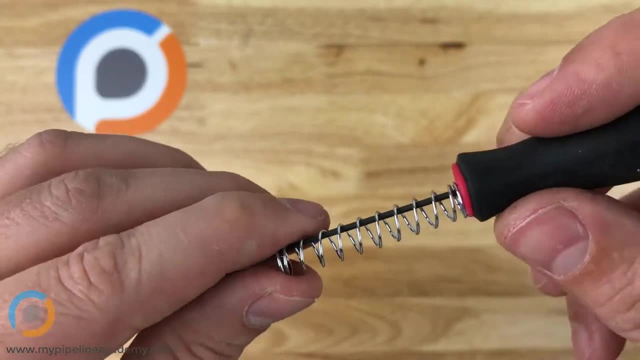 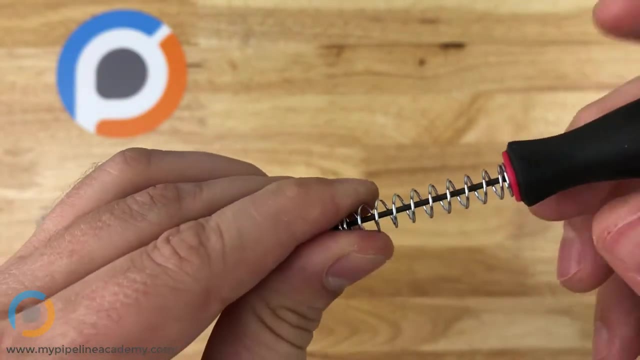 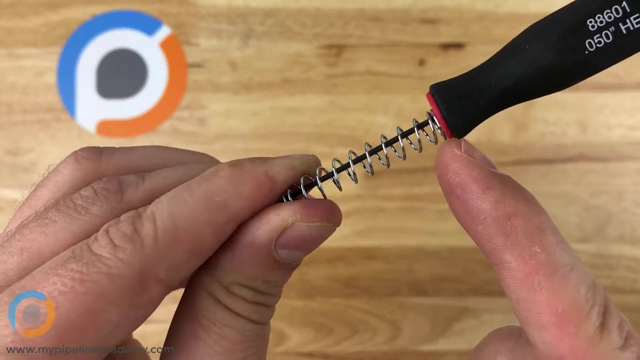 Our low-tech solution was to use a spring and then calculate at what amount of compression we'd get two pounds of force. and then we we just made a marking on the other part, and that marking corresponded to the amount of deflection. so if our pushing starts right, here we maybe we had a.